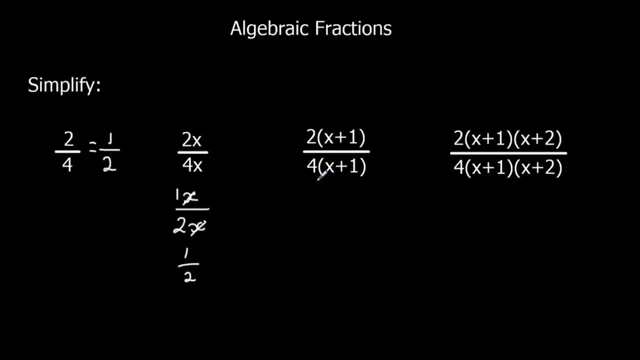 well, Here I've got x plus 1 and x plus 1.. So I can divide the top and bottom by x plus 1.. So that will cancel them out. So I'll get 2 over 4, and if I divide top and bottom by, 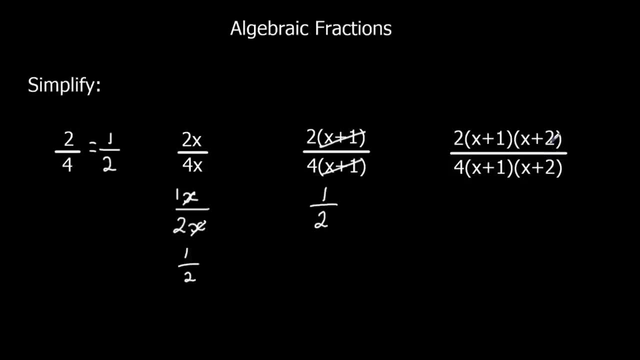 2, I'll get 1 over 2.. And finally, here I've got. I can divide top and bottom by x plus 2.. Divide top and bottom by x plus 1.. And half the top and the bottom again. So all of these fractions here are. 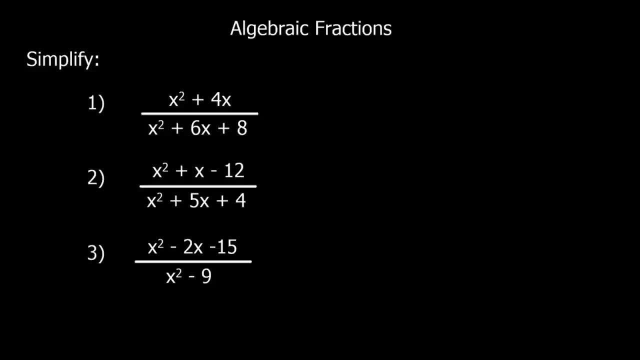 the same and they just mean half Okay, so in this case it doesn't look like we can divide the top and the bottom by the same thing. What you definitely don't do is: you don't go. they've both got x squared. 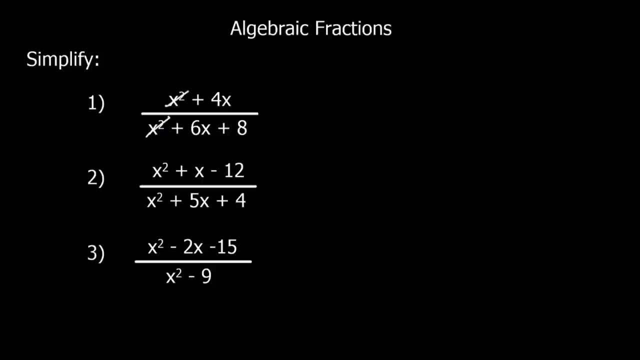 because that's not dividing by x squared, that's taking x squared off, And we can't do that. So what we've got to do here, the first step, is we've got to put them into brackets, So we've got to factorise the top and the bottom. So let's have a go at that. 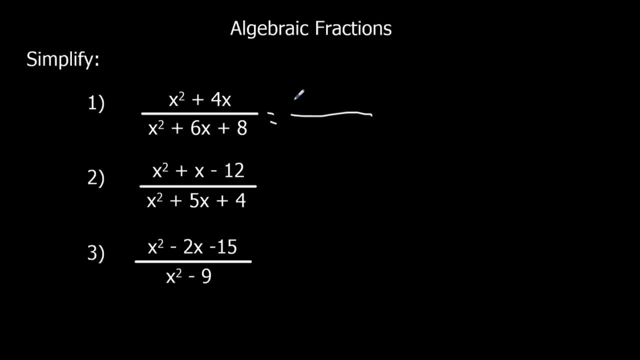 So we're going to do what's in both of these x, so we'll have x, x plus 4.. And then double brackets on the bottom, x in both. What times is to give 8? And add to give 6, plus 2, plus 4.. Now we could have known. we. 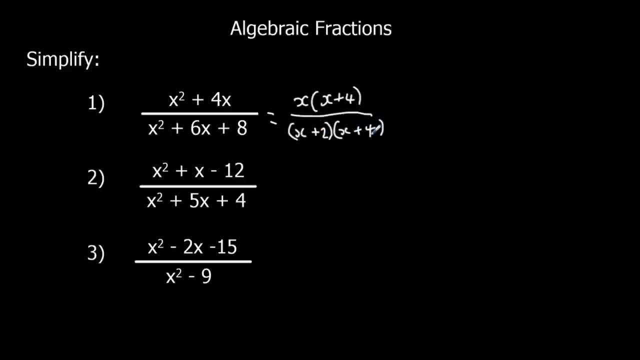 could have guessed it was going to be a plus 4, because we needed that to cancel out. And we can divide top and bottom by x plus 4, and that leaves us with x over x plus 2.. We can't simplify this anymore, because we can't divide top and bottom by the same thing. So 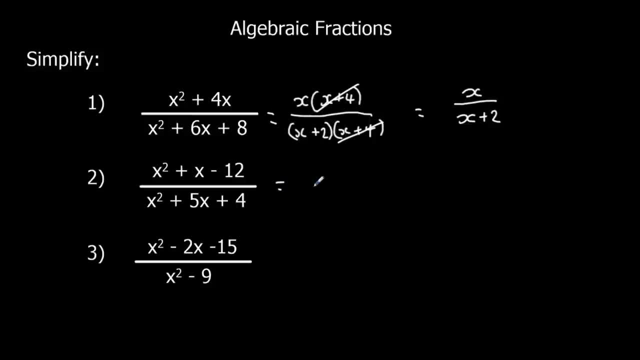 that's the final answer. Okay, same again here. we need to factorise the top, factorise the bottom, So they're both double brackets. What times to make 12, and add to make 1? A, b plus 4. 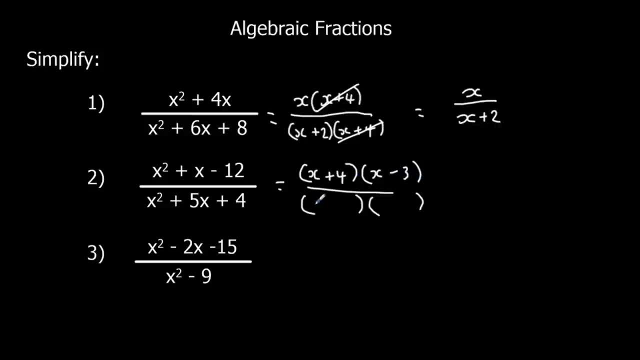 minus 3.. And on the bottom, we know one of these two is going to be in it. What times to make 4, add to make 5,, 4 and 1. And we cancel out the x plus 4s. So the final answer.